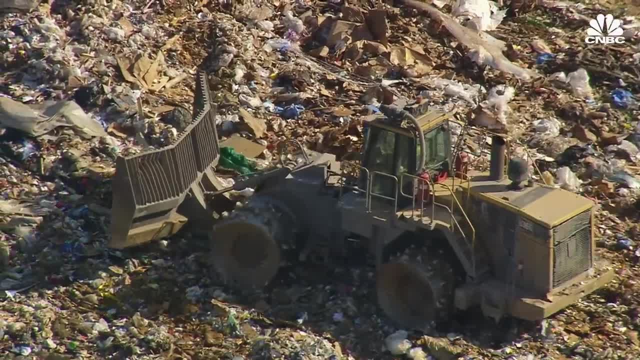 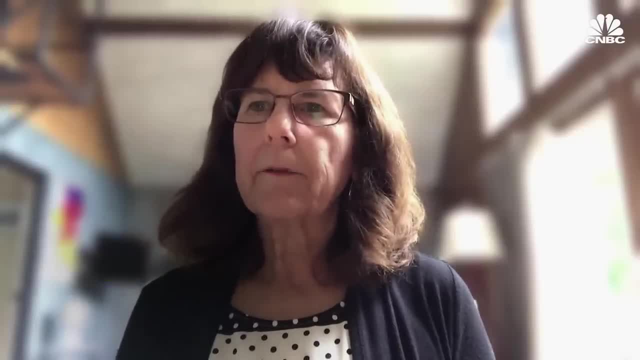 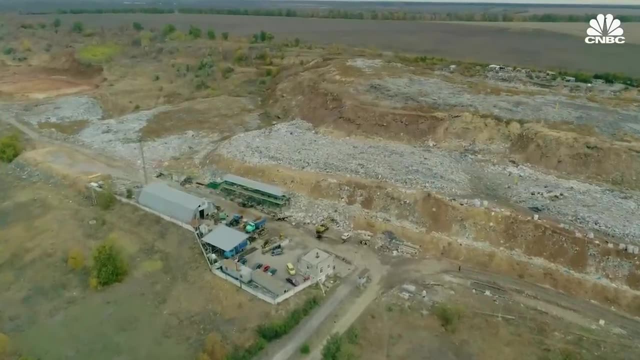 It's a profitable industry. It's a difficult industry, but it is profitable. It's done right, And I think that is why there are so many private companies That are involved in waste management. Thanks to advancements in modern chemistry and the support from the government, landfills have seen astonishing financial success in recent years, raking in millions of dollars in profit. 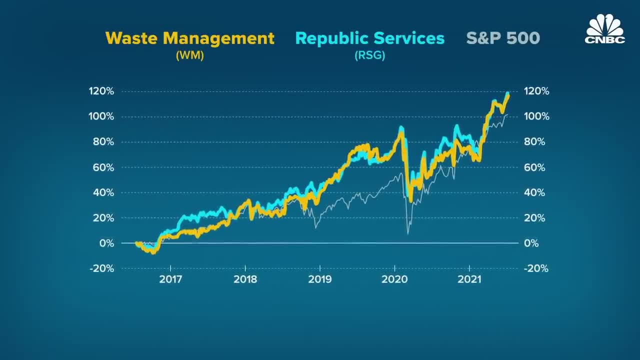 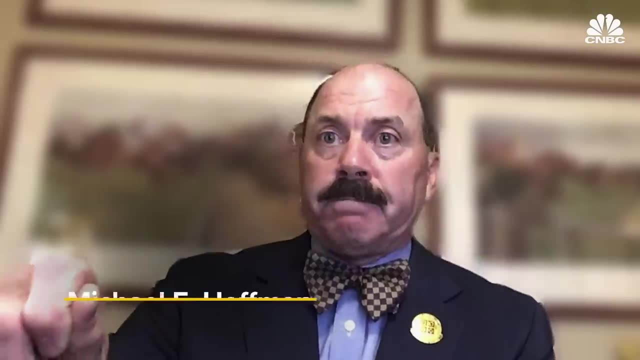 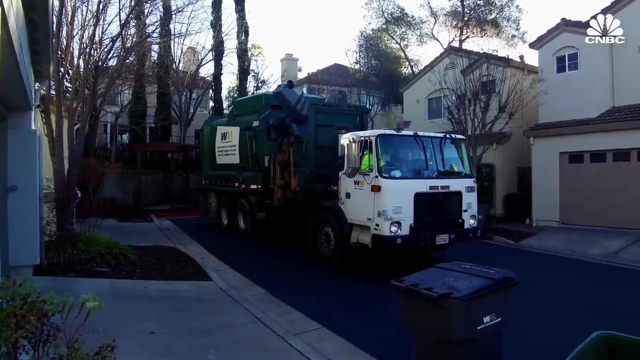 Private solid waste management companies like Waste Management and Republic Services have shown significant growth over the last five years. They've learned how to be best in class businesses And, as they did that, what you saw was this growth occurring in new customer growth, new business formation linked with consumerism, consumer engagement. 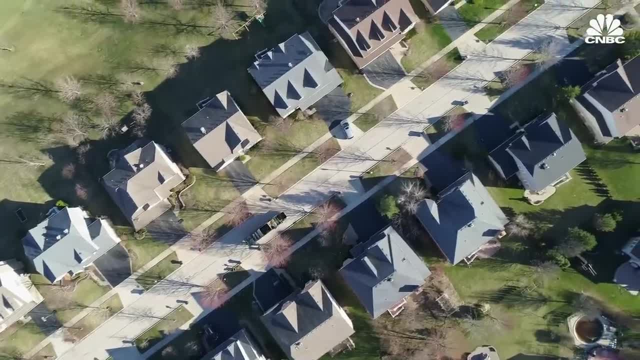 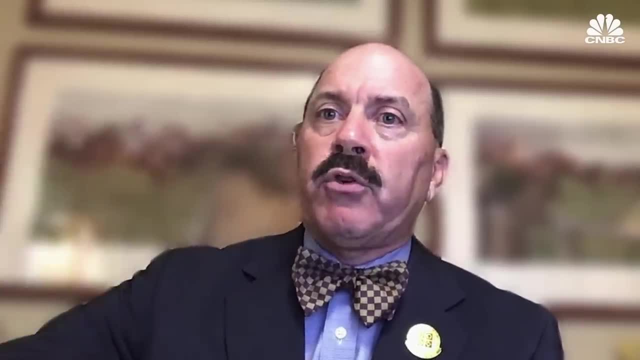 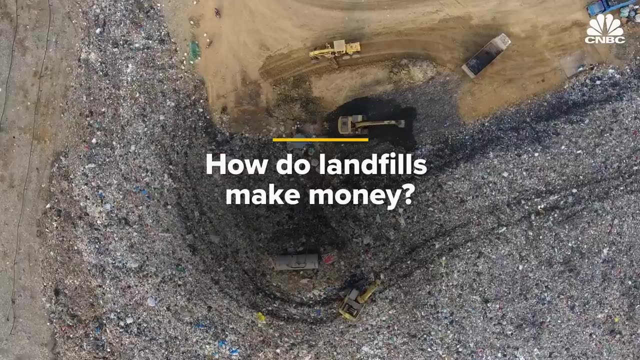 Housing and the garbage industry. publicly traded stocks outperform the market handily between 2015 and 2019.. And underpinning it is a meaningful improvement in their free cash flow conversion. So how exactly are landfills turning profit out of garbage and just how much money can be made? 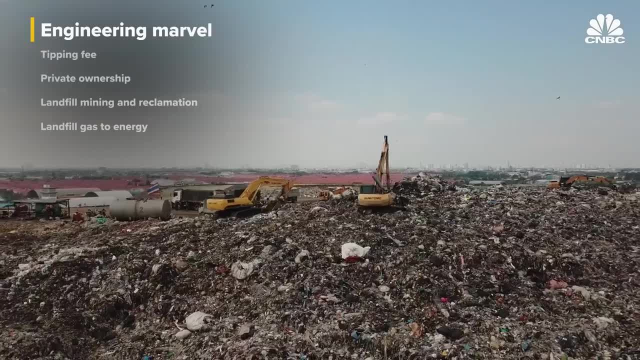 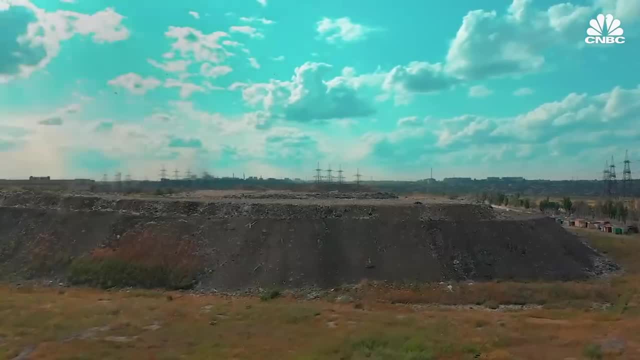 When people think of landfills they usually imagine an endless field of garbage emitting a terrible odor and housing all manner of pests. But modern sanitary landfills today Are much more nuanced and a lot less smelly. A modern landfill is a civil engineering marvel. 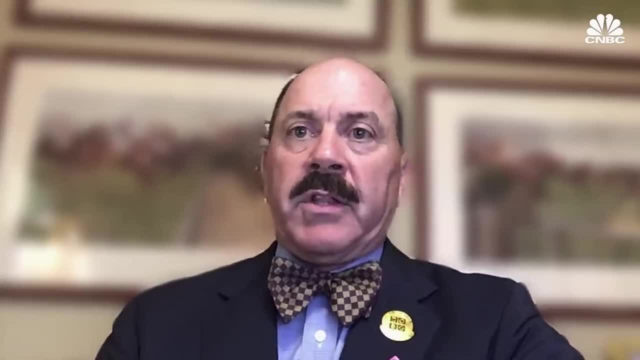 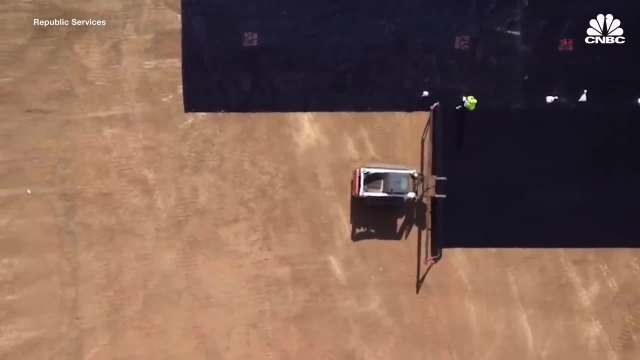 These are extraordinarily well engineered. They're designed to protect human health and the environment and, at the same time, contain and manage the waste that we generate at four and a half pounds a person per day in the United States. If you walk past the landfill and there is a smell, that means they are doing something wrong. 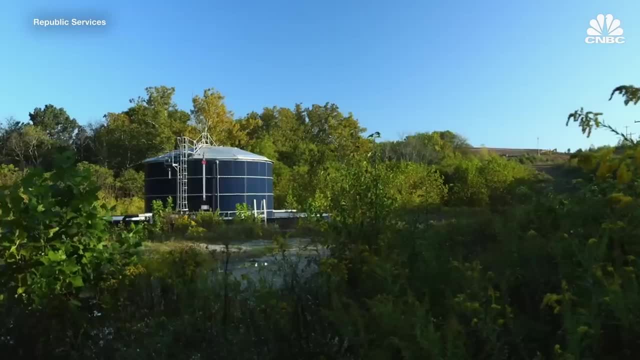 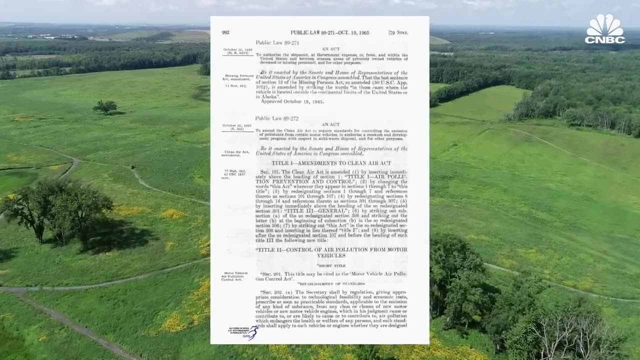 Strict regulations and the work by the EPA have changed landfills to become more modern and sanitary than ever. The Solid Waste Disposal Act of 1965, combined with the Resource Conservation and Recovery Act of 1976, dramatically expanded the federal government's role in managing waste disposal. 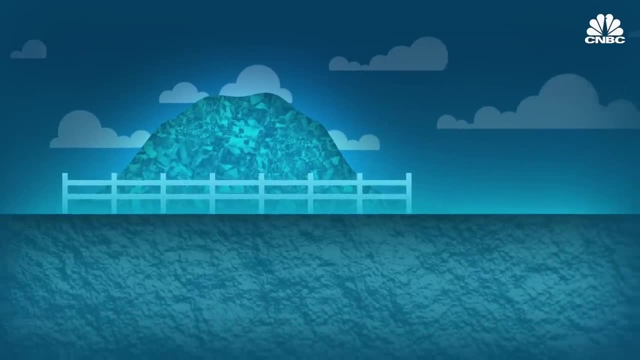 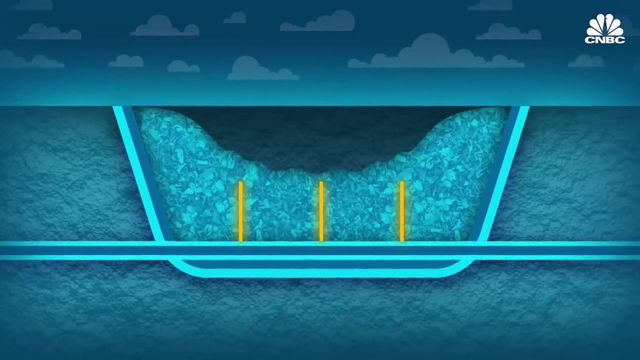 Open dumps, where garbage is dropped off without any protection, are now illegal. When waste is brought to a sanitary landfill, they are disposed into an open section known as the cell. This cell is protected by a layer of reinforced plastic, known as the liner, that prevents any harmful liquids from leaking out. 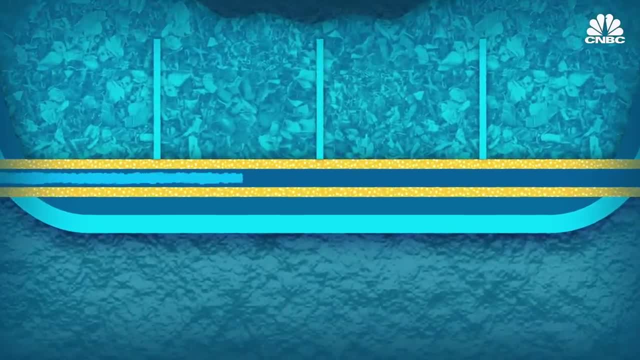 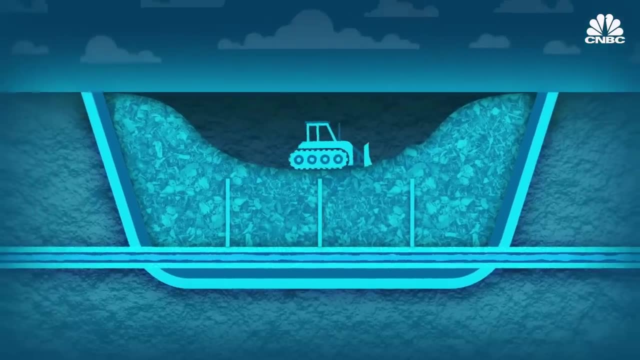 Any liquid from the landfill is removed from. the waste is collected at the bottom of the landfill and is removed via a series of pipes, gravels and sand. Meanwhile, above ground trash is constantly compressed within the cell using bulldozers and other compaction equipment. using daily 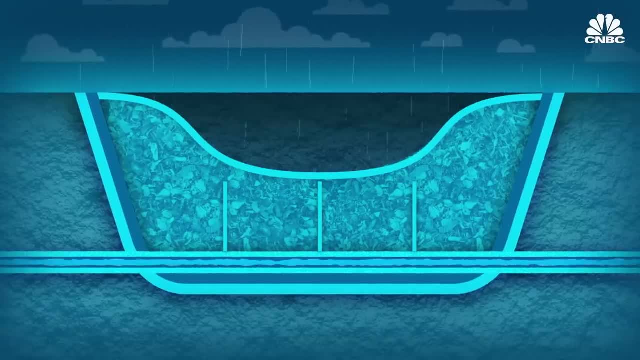 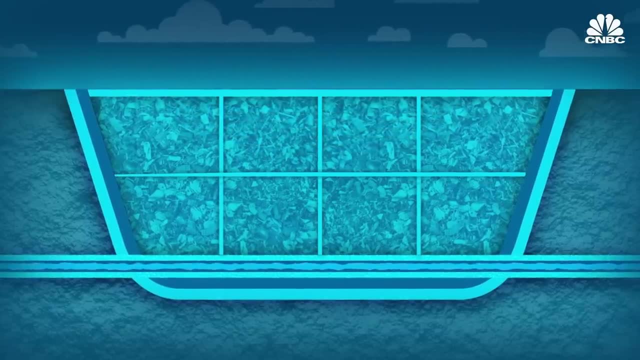 covers to protect the trash from sun, rain and pests until the cell reaches its max capacity. Once that happens, either a new cell begins on top or a final cover is placed over. The site is then continuously monitored for up to 30 years to ensure. 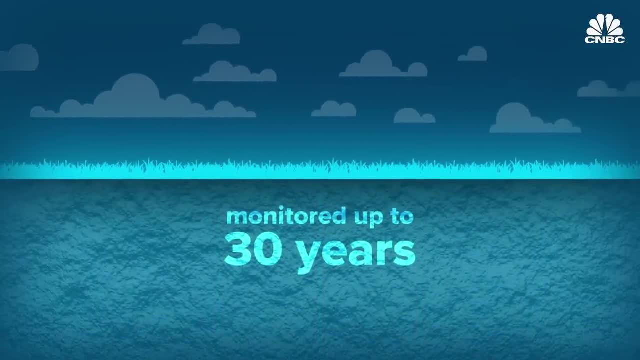 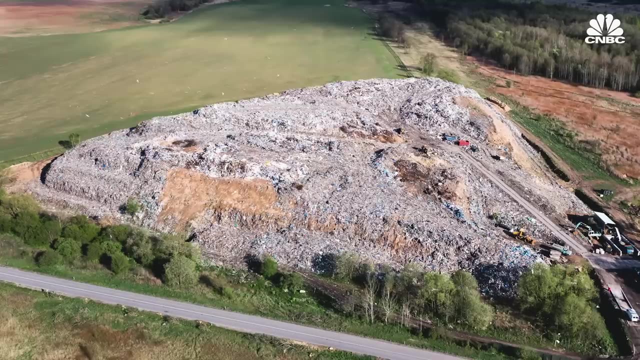 everything is environmentally sound. There is the potential for the liner system to leak, for example, over long periods of time, and probably more likely the cover system. you know, it's just going to be subject to that settling and weathering and different things. So there's the potential. 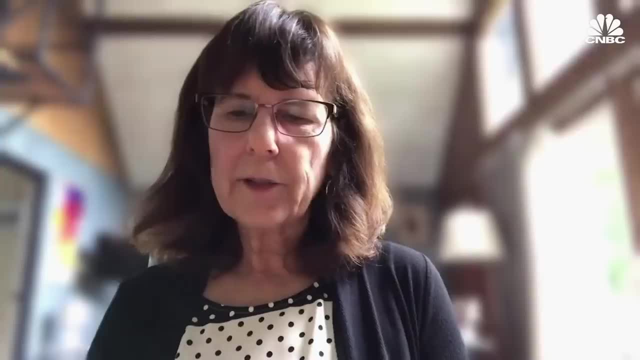 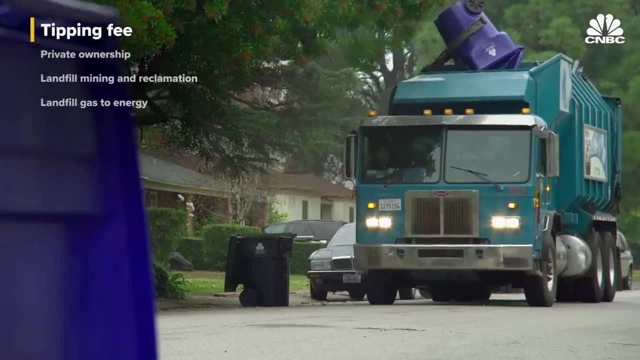 for gas emissions. You want to be monitoring a landfill. as long as there's the potential for gas or liquid emissions, Landfills make a majority of their revenue even before the garbage makes its way to the pile of trash Through a tipping fee or a gate fee. 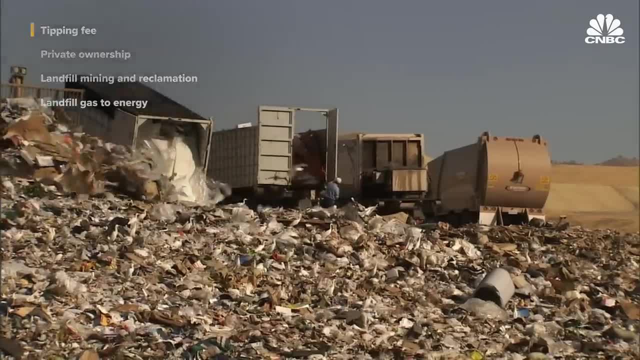 landfills are able to collect and dispose of the garbage. landfills are able to collect and dispose of the garbage. landfills are able to collect and dispose of the garbage. Landfills charge trucks dropping off their garbage based on their weight per ton. This fee acts as the lifeblood of most. 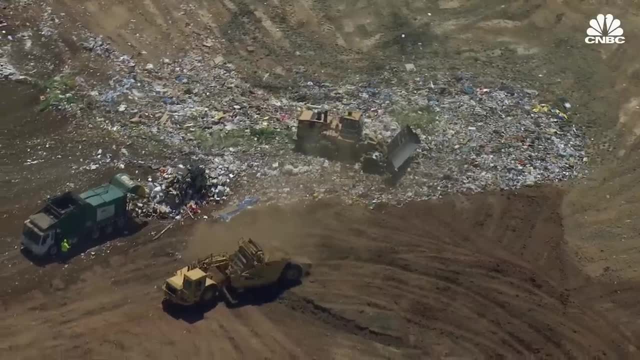 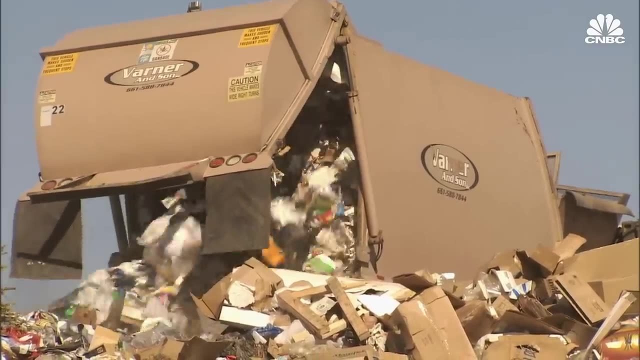 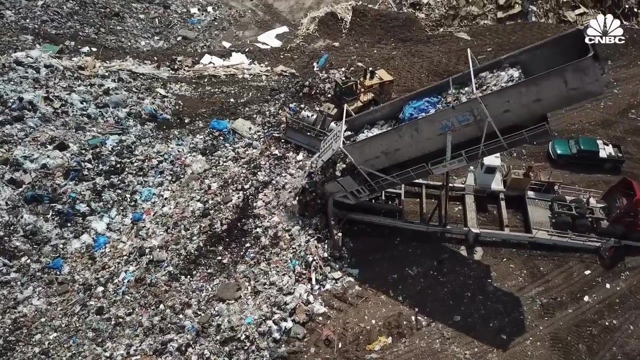 landfills across the United States. Tipping fee gets its connotation because the truck comes in and tips, if you will, and it literally tips up when the trash is driven out of the trailer through what's known as a walking floor. So tipping is, it's your pay grade, It's the 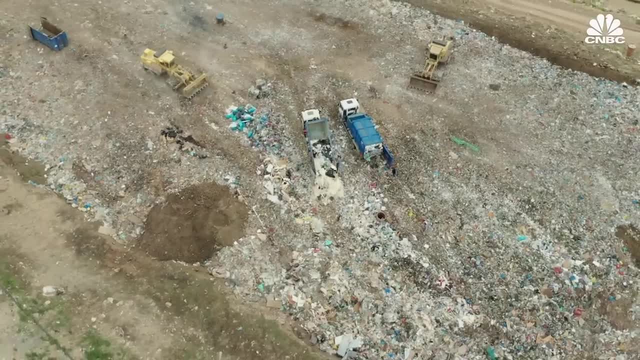 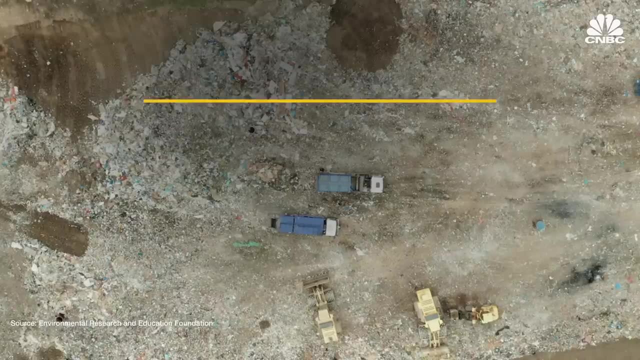 price per ton And that is the principal source of income. In 2020, municipal solid waste landfills had an average tipping of $53.72 per ton. That translates to roughly 1.4 million a year in approximate average gross revenue for small landfills and 43.5 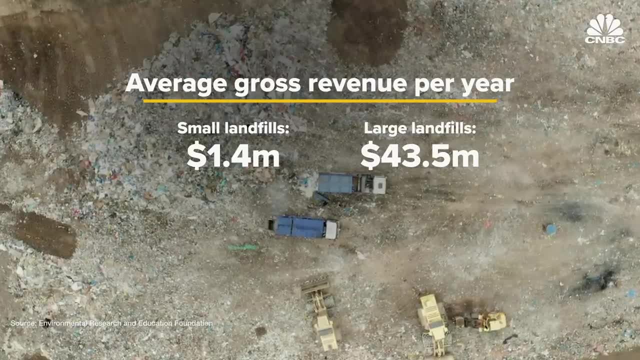 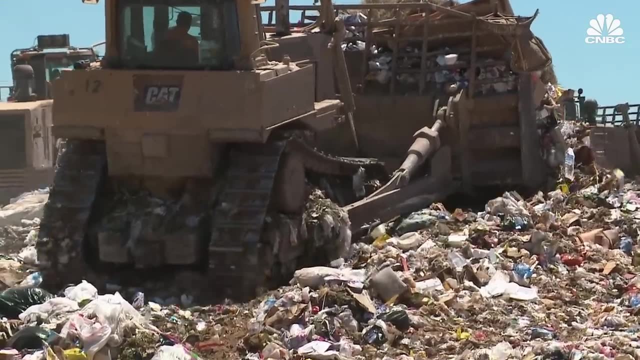 million a year for large landfills. just from gate fees And tipping fees have seen steady growth over the past four decades. In 1982, the national average tipping fee sat at $8.07 per ton, or about $23 when adjusted for inflation. That's. 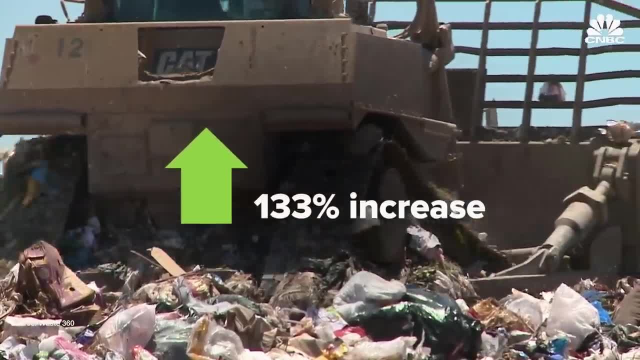 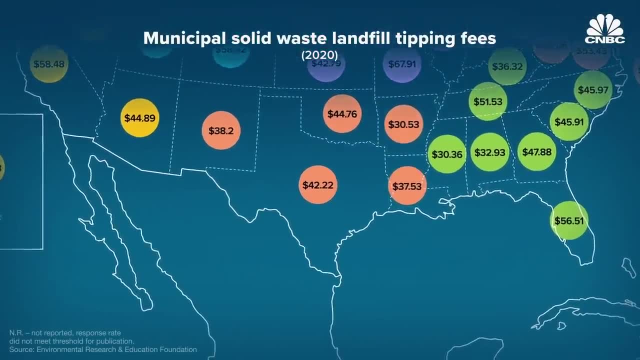 nearly a 133% increase in the average gross revenue per ton. Tipping fees vary widely depending on where the landfill is located. For instance, the South Central region in the US has the lowest average tipping fee, of $39.66 per ton, with some states. 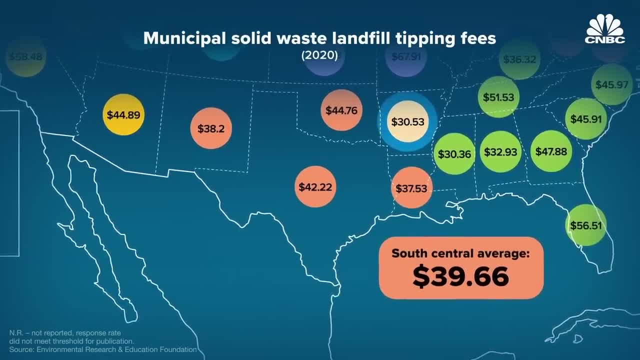 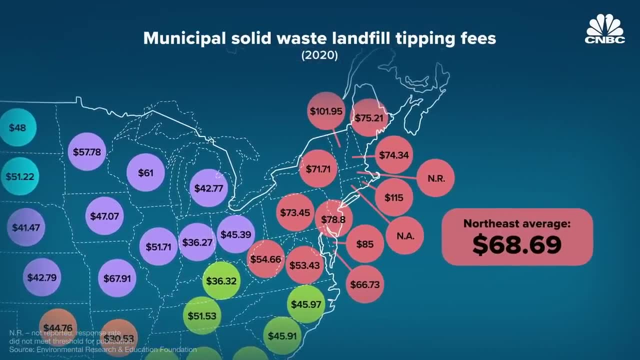 like Arkansas, reporting a fee as low as $30.53 per ton. On the other hand, the average tipping fee in the Northeast is almost double that at $68.69 per ton, with states like Delaware reporting a fee as high as $85 per ton. 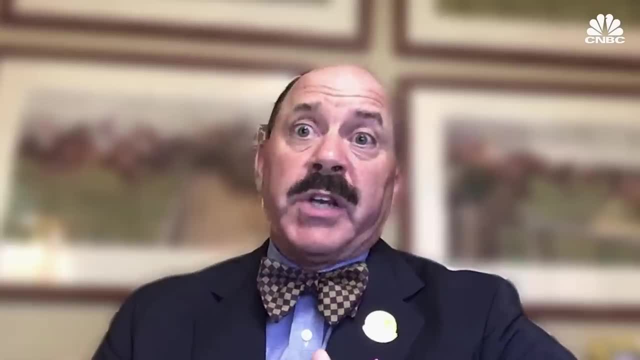 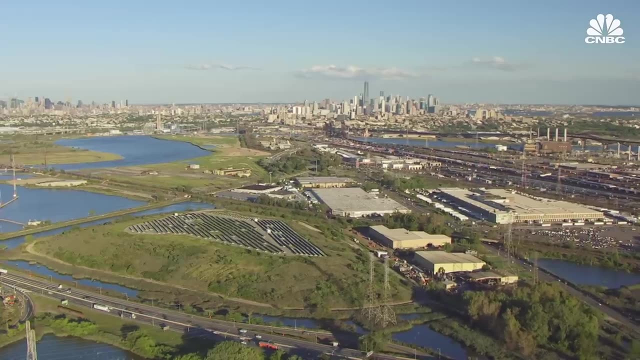 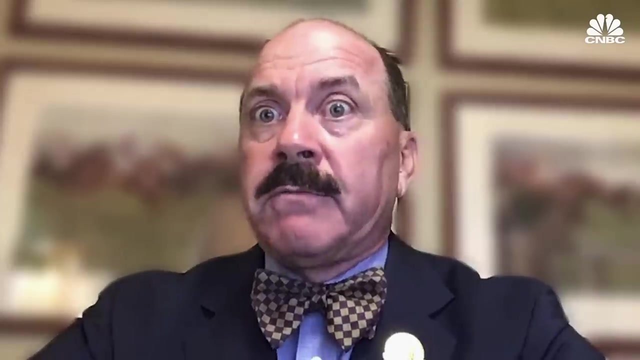 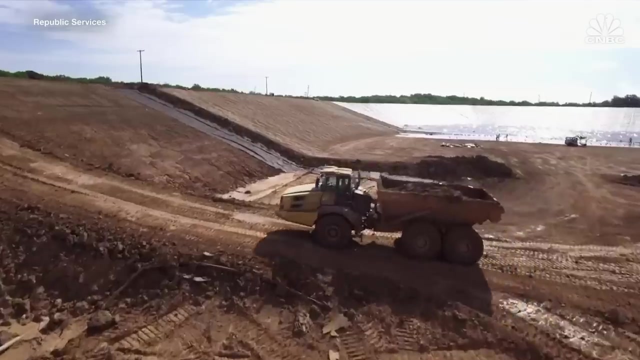 The list of reasons, but at its simplest level is scarcity. So where tipping fees are the highest, I would venture that you have extraordinarily dense populations and very few disposal options. The other difference is the cost of building. If I'm in Western Pennsylvania dealing with rock formations at very shallow 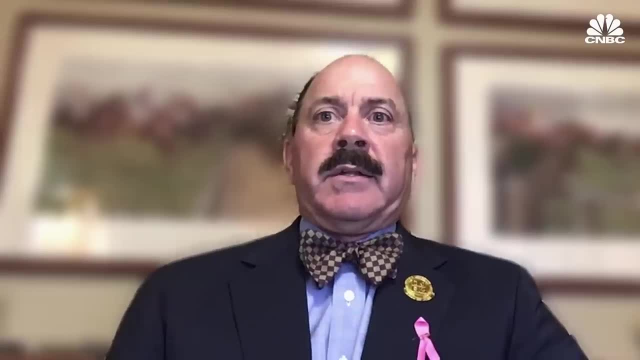 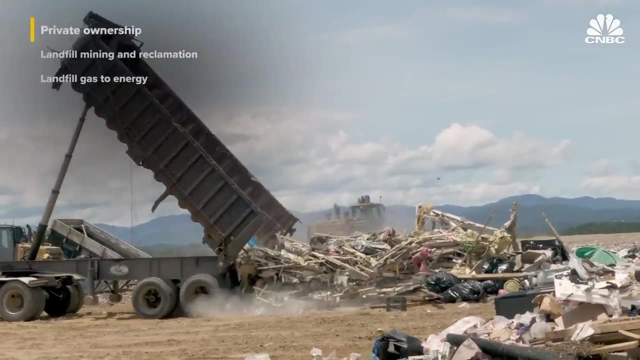 level, and then I literally go 50 miles west and go to Ohio. the cost of building a landfill in Western Pennsylvania versus Ohio are dramatically different. While tipping fees make landfills sound like a risk-free business, they are still quite an expensive investment. It can cost about $1.1. 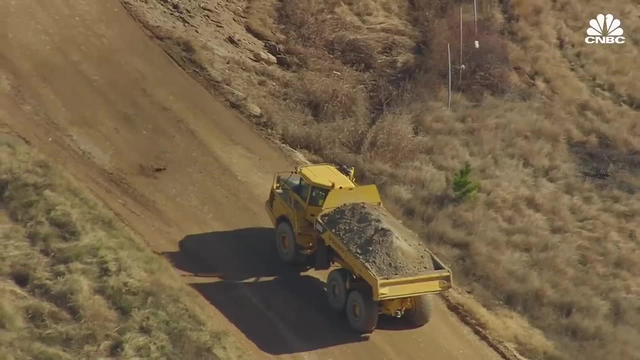 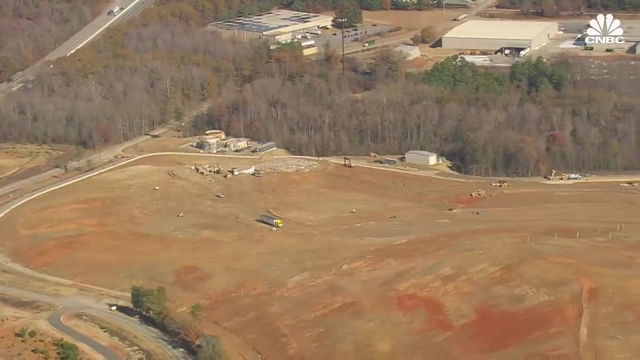 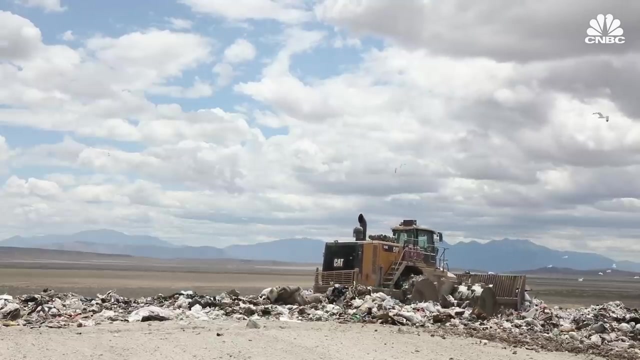 to $1.7 million just to construct, operate and close a landfill And there are financial obligations that must be met even after the landfill has been closed entirely. There was a major regulatory change that happened in the 70s, called the Resource Conservation Recovery Act. By 1994, every landfill in the 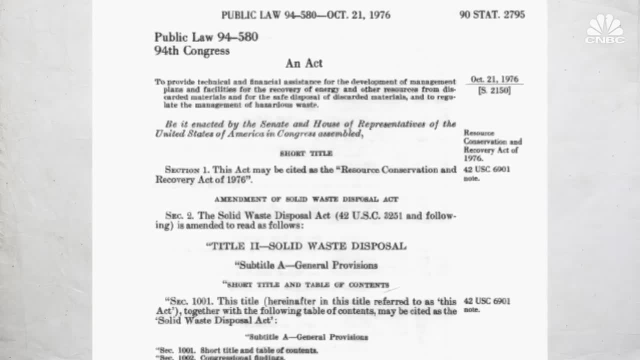 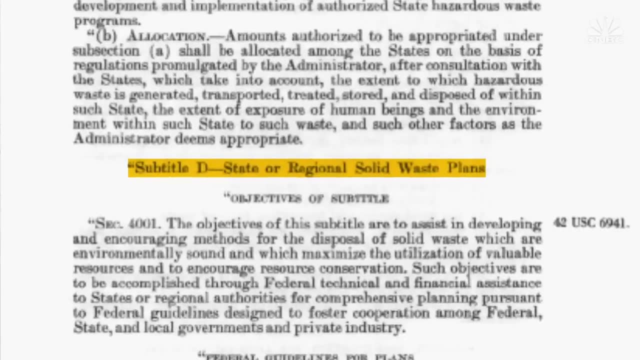 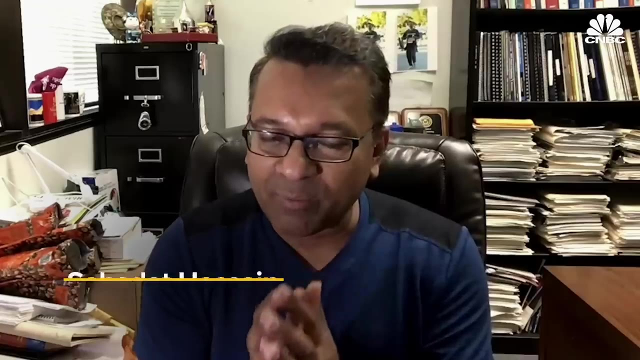 landfill that was in service in North America had to adhere to something called Subtitle D, which is the design operation and then the lifecycle financial assurance obligations of managing and overseeing that site for 30 years after it closes. So every business owner, whoever owns the business they make, money up to the time it's working. Then, even after closing, they have to pay the maintenance fee, which is around $1 million without making money for 30 years. That's part of their business operation, So they need to make money after. 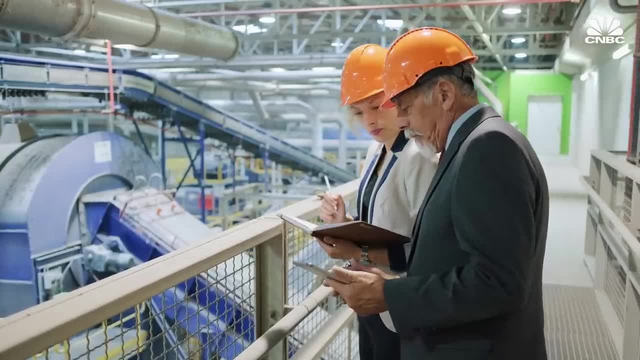 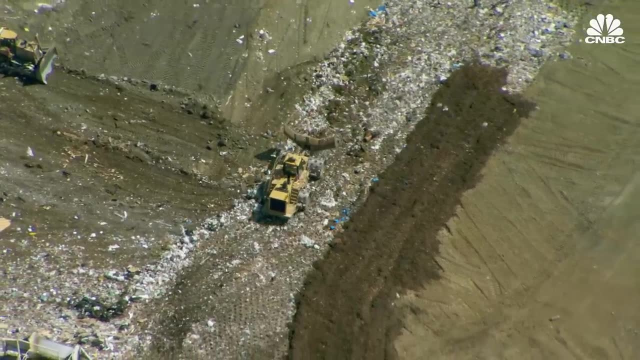 Today, private companies have replaced municipal governments to own and operate the majority of landfills across the US. In 1988, about 7,900 landfills were publicly owned. By 2009,, that number had fallen to about 1,900.. 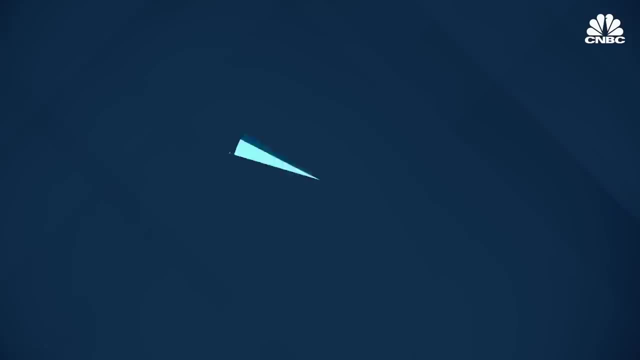 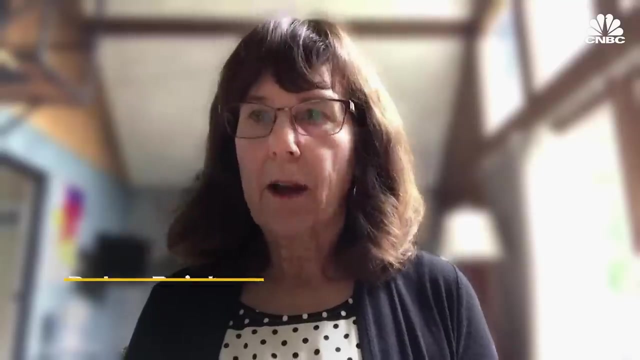 It's now estimated that more than half of all municipal solid waste landfills are privately owned, with the industry controlling 85 to 90 percent of permitted capacity. Landfills are often owned by private companies, and I think it's because the trend has been to go larger and larger. 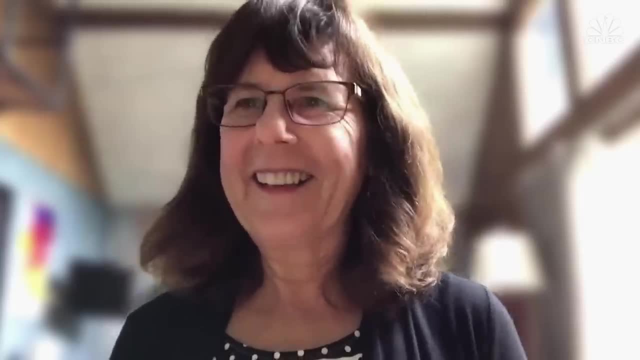 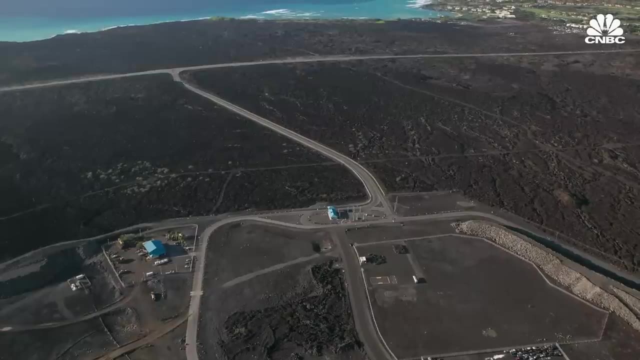 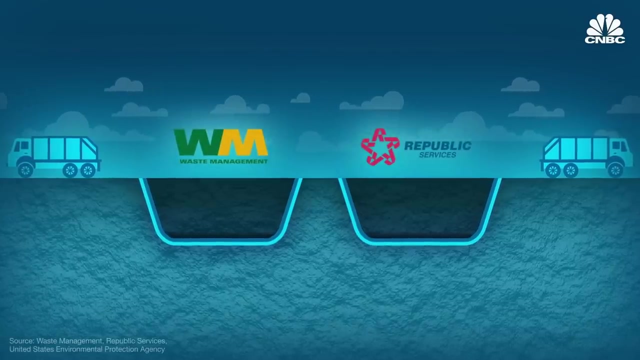 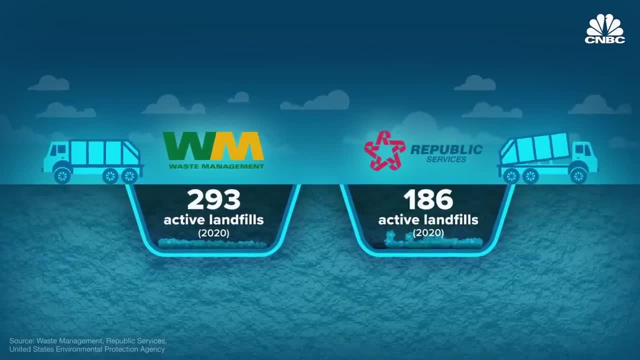 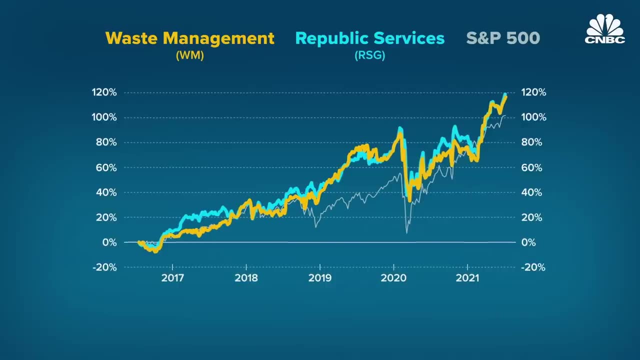 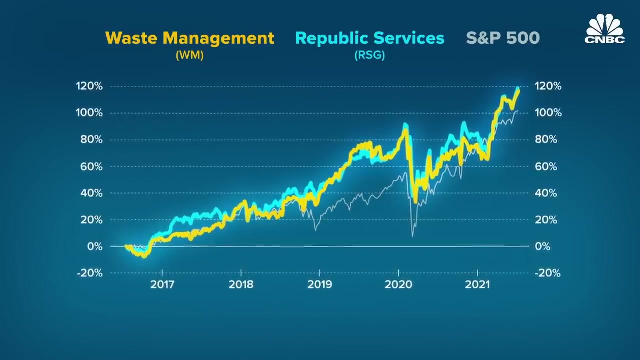 US, While Republic Services says it operates just over 180 out of the 2,627 landfills across America. Together the two companies have seen staggering performance in the market, with both companies stock prices doubling in the past five years. If you take the great recession and sort of lay the framework of how 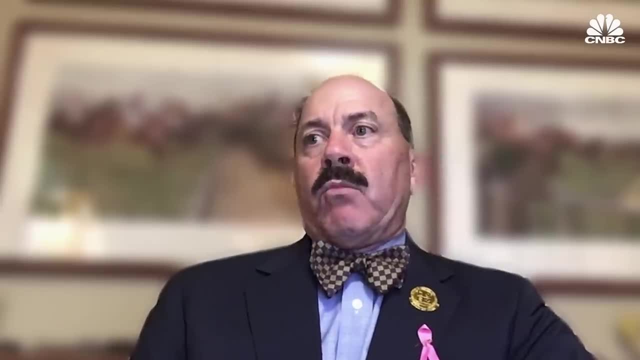 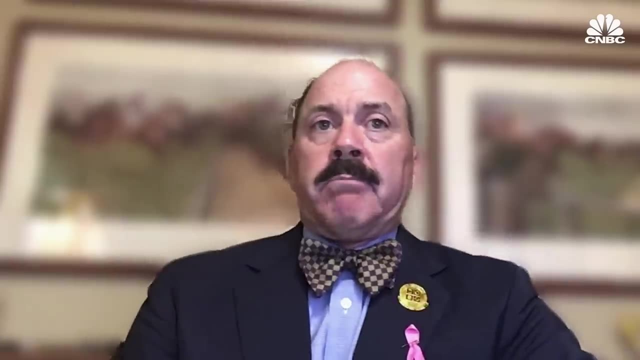 to garbage, perform. post the great recession. what you'll discover is there's a five year window window up to 2014,. where they did okay, they were. you know they're in the green, matching or slightly outperforming the. 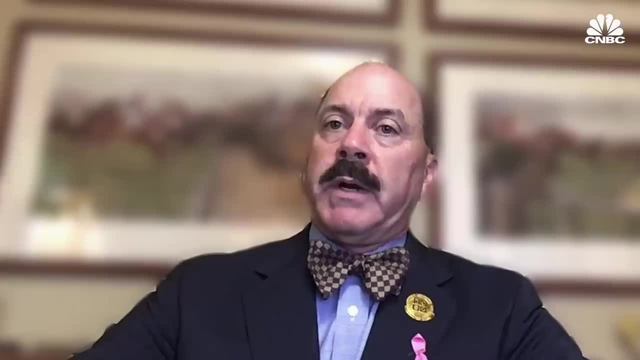 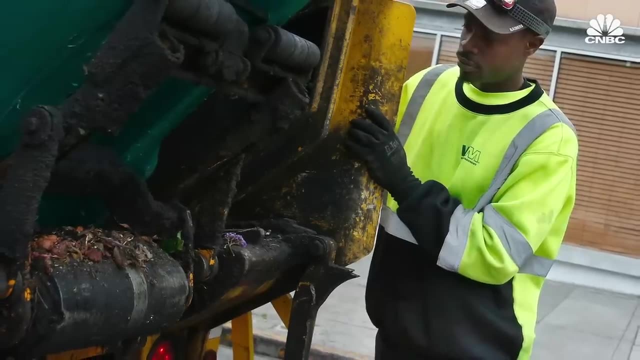 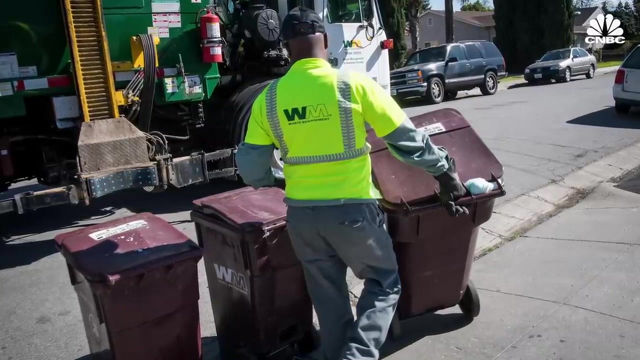 market, but the significant outperformance begins in 2014 through 2019.. They've learned how to be best in class businesses And, as they did that, what you saw was this growth occurring in new customer growth, new business formation linked with consumerism, consumer engagement, housing and the garbage industry. publicly traded stocks outperform the market handily between 2015 and 2019.. And underpinning it, is a meaningful improvement in their free cash flow conversion. Some government jurisdictions have also transitioned to a hybrid ownership In places like Wake County, North Carolina. 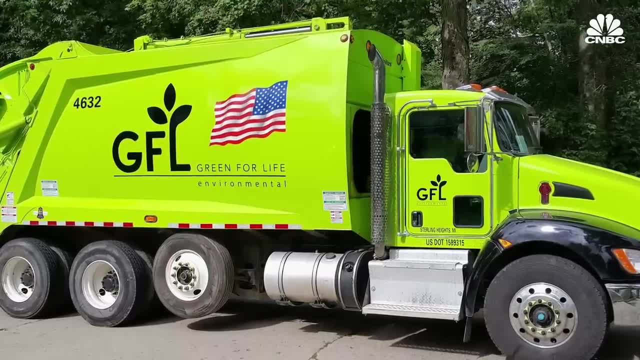 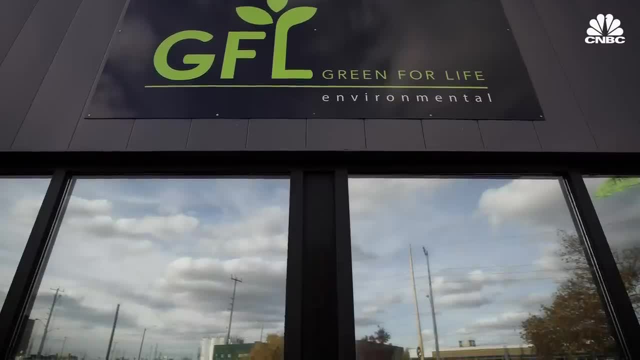 landfills are owned by the county but operated by GFL Environmental, a private company. So if you give it fully privatized, a private company will try to go through the regulation, but the main focus would be making money. To me, the combination of both is the best. 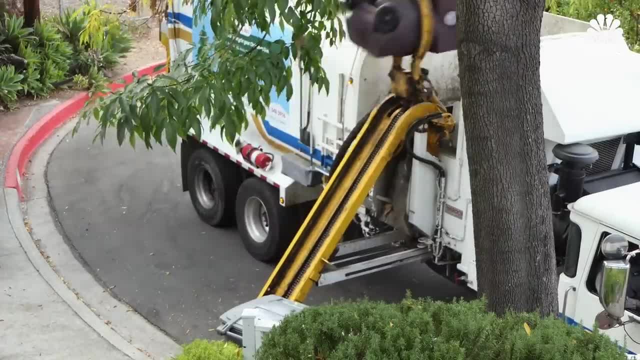 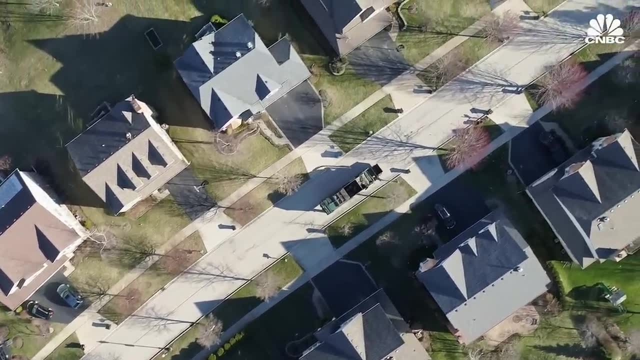 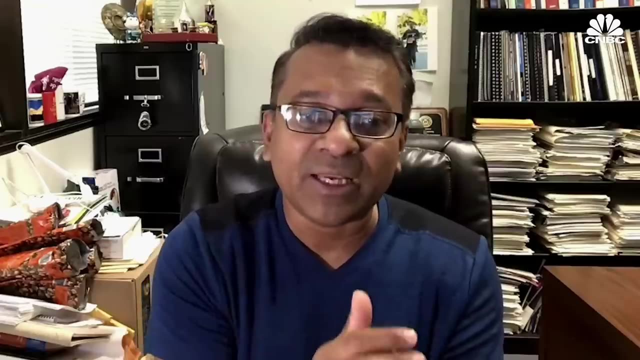 choice, Because that way city has certain control over the landfill company. they will look at only for the profit. But city also needs to make sure that not only the profit, the environmental sustainability, environmental cases and people's life, the case, everything is maintained in the right way. 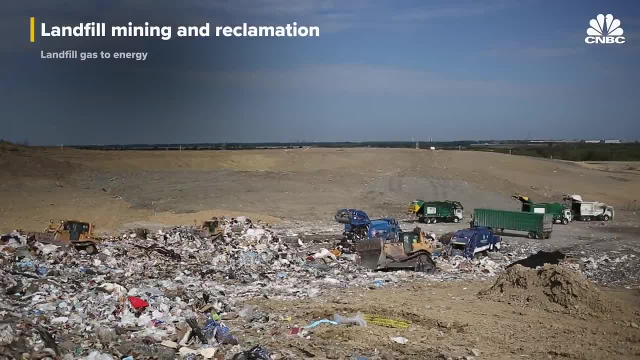 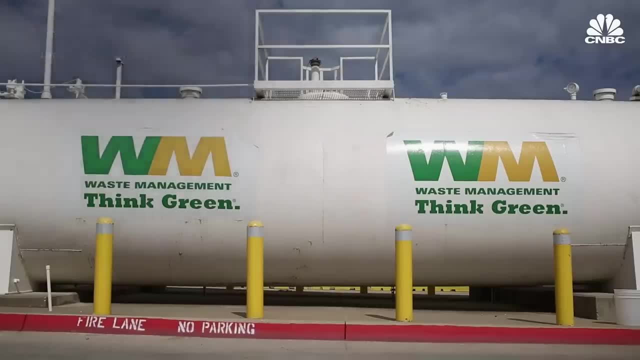 Private companies have also discovered new ways, beyond tipping fees, to turn profit out of their garbage. Landfill mining and reclamation, a process of extracting and reprocessing materials from older landfills, is one of the most common ways to save money, And it's a way to save money. 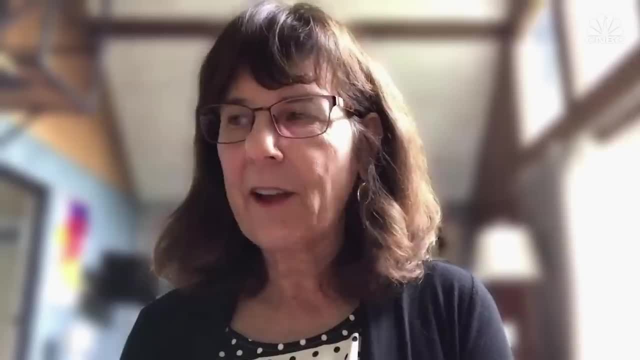 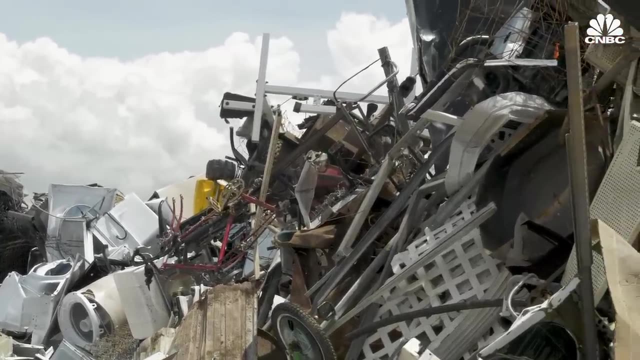 And it's a way to save money. And it's a way to save money. Certainly, looking at waste as a resource is the best thing for the economy. It's the best thing for the environment, for health. Putting metal in a landfill just makes absolutely no sense. 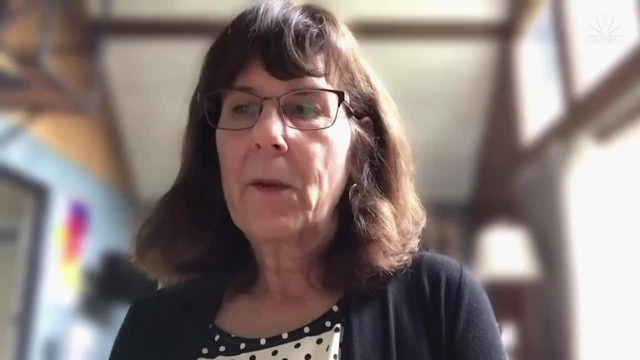 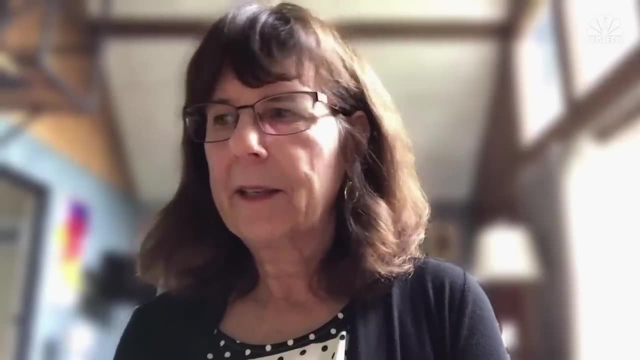 It's just going to sit in the landfill forever and ever and ever. There'll be some corrosion, but it's pretty much going to sit there, Whereas metals are so easy to recover and recycle and save so much money and energy and so forth. In 2017, a private scrap metal company contracted with a nonprofit landfill in southern Maine to mine precious metals. In four years, they recovered over 37,000 tons of metal worth $7.42 million. But it isn't always a success story. 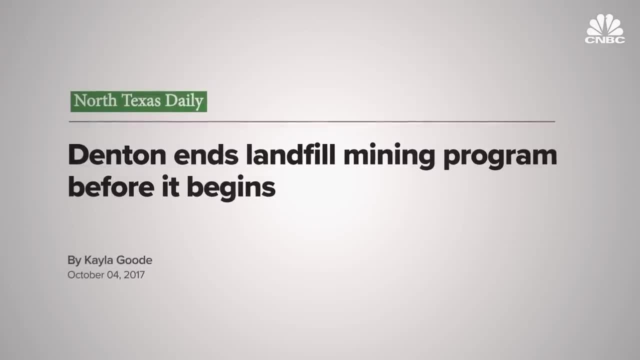 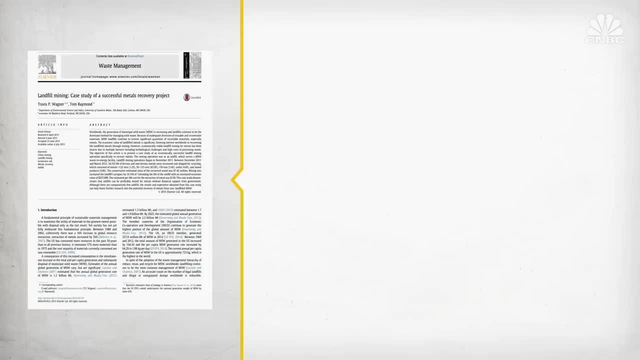 In 2017, the city of Denton, Texas, ended their landfill mining program before it could even start, after realizing that the benefits weren't worth its $4.56 million price tag. According to experts, economics is usually the biggest challenge to make landfill mining work. 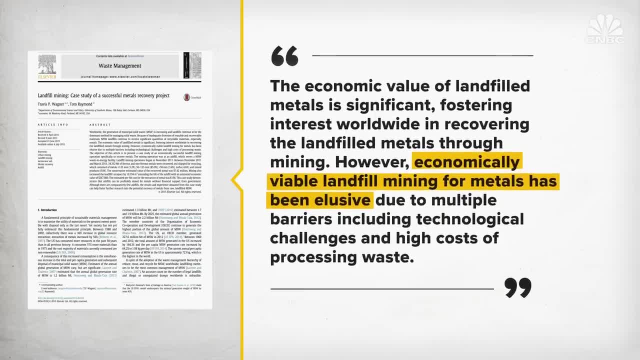 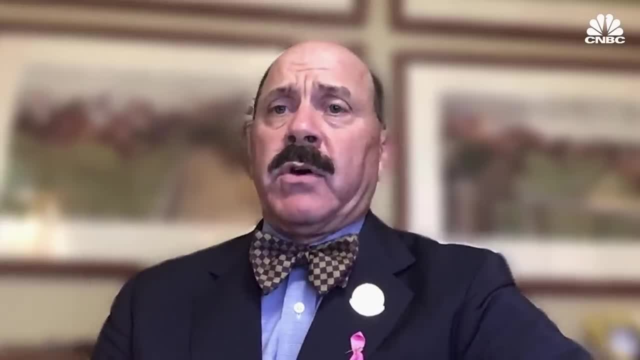 There's virtually no way I can see how that makes money. The commodity values would have to be at such higher levels than they are today, Whatever it is you're trying to get your hands on. However, some experts claim that landfill mining can be profitable. 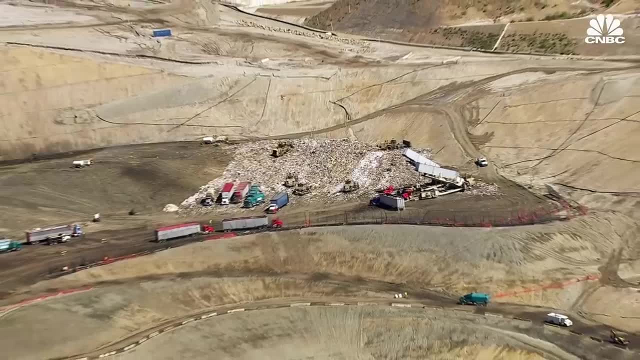 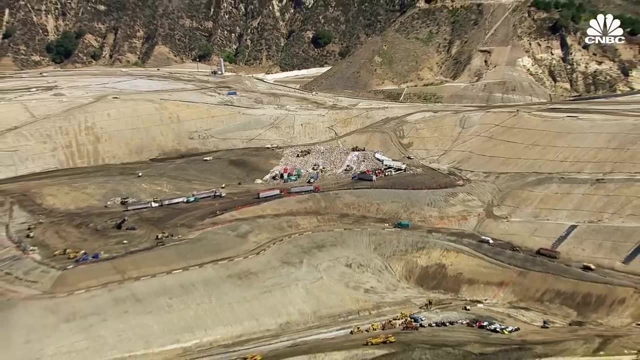 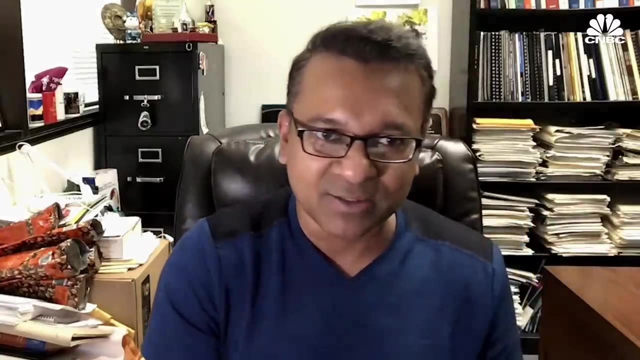 if done correctly. That's because mining can often recover the most valuable asset of any privately owned landfill space. You get new tipping fee right, You put the trash back into that mine. You build a new landfill without buying a new space, So that space gives you a lot of money when you start backfilling. 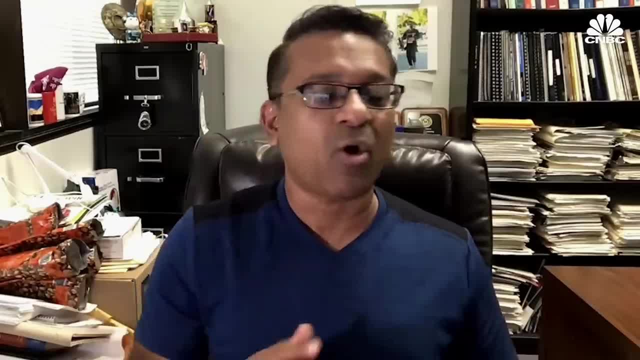 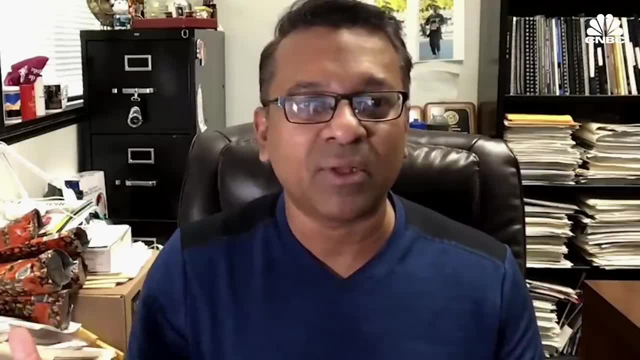 Many people are mining but they're not reusing the space. So they're saying, oh OK, we cannot make money out of mining. Yes, you cannot, But if you do the operation right, you're never going to be involved. 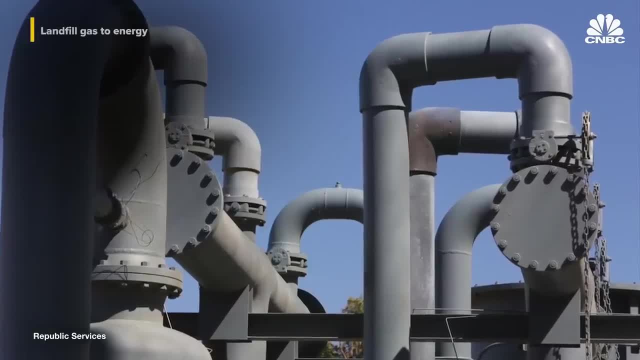 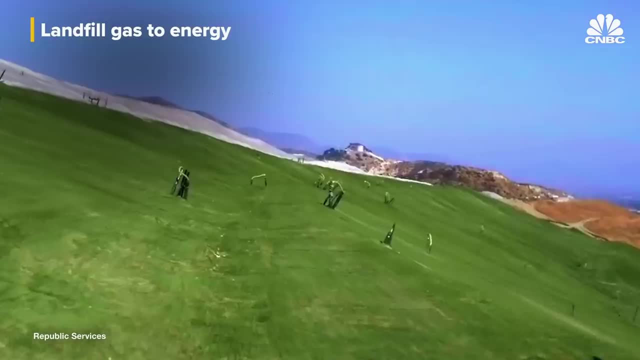 You will always make money. Modern chemistry has also allowed landfills to be mined for energy. When trash decays inside a landfill, it's a waste of energy. It produces methane gas. For decades, regulations have required landfills to suck out this. 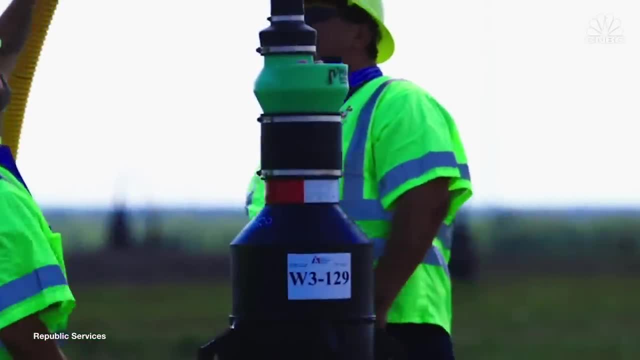 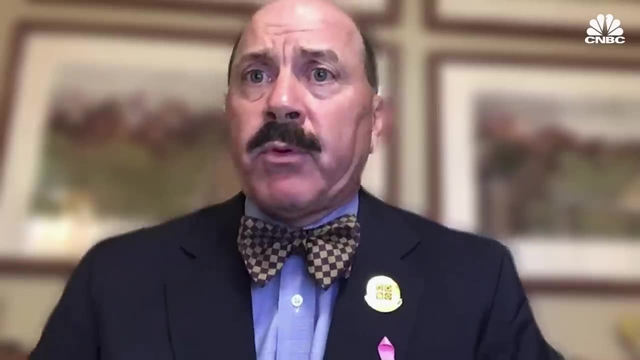 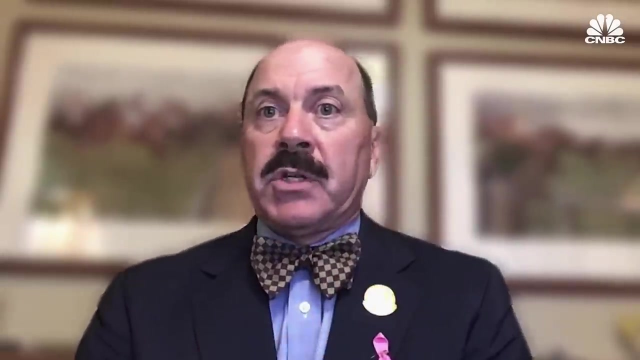 highly flammable gas and dispose of it safely. Landfill gas to energy projects, however, use the same gas to produce fuel and generate electricity for profit. The landfill gas operations that are known as low or medium BTU, which are a predominant form of capture the gas- polish it a little bit- turn. 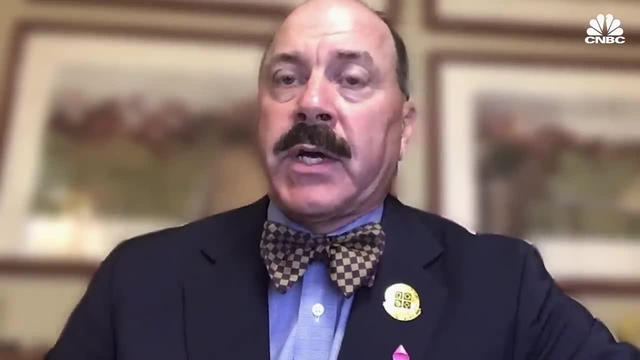 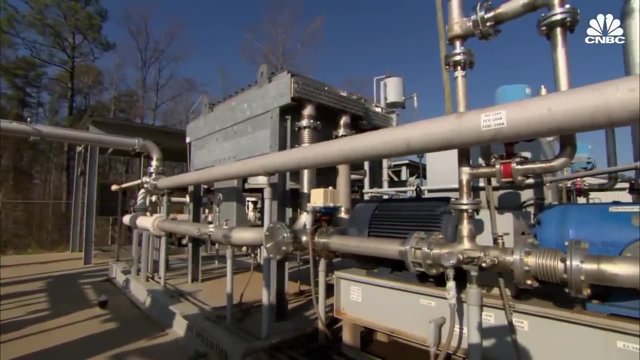 it into electricity or steam and then sell it. Those are good return on capital projects. According to the US Energy Information Administration, Landfill gas generates about 10.5 billion kilowatt hours of electricity every year. That's enough to power roughly 810,000 homes and heat nearly. 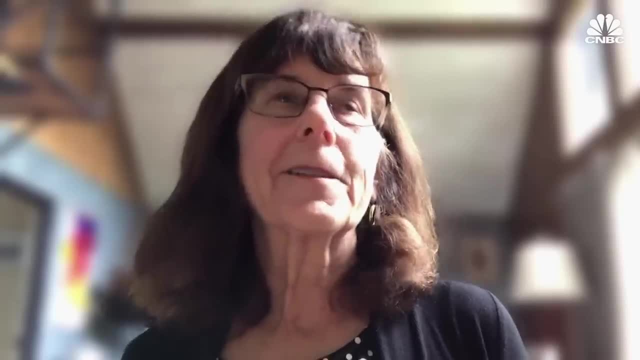 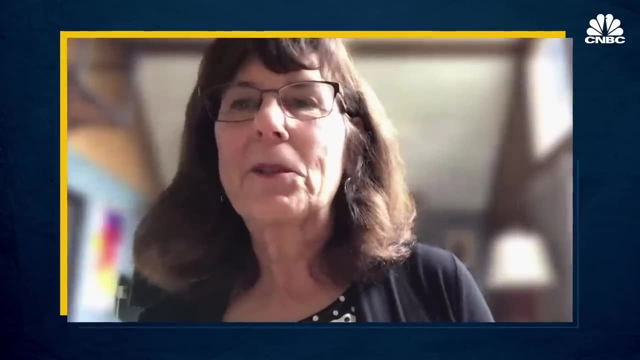 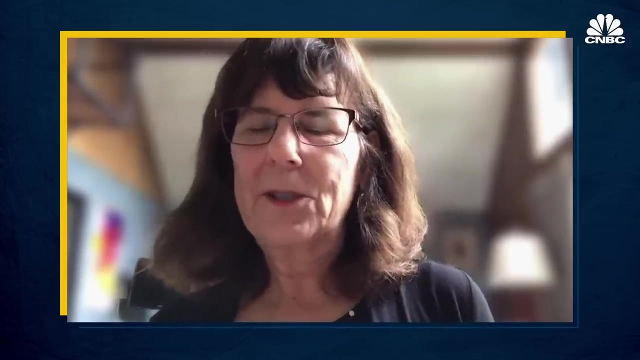 540,000 homes each year. I just did a paper where I was looking at how much electricity you can generate from landfills compared to how much energy we're using to produce electricity, And it's like less than 1 percent. I mean, it's a minor contributor to our heavy demands. 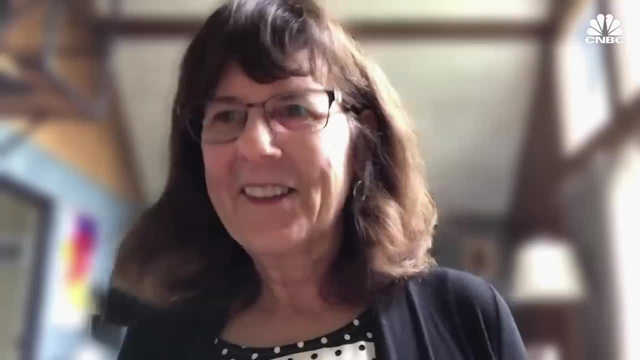 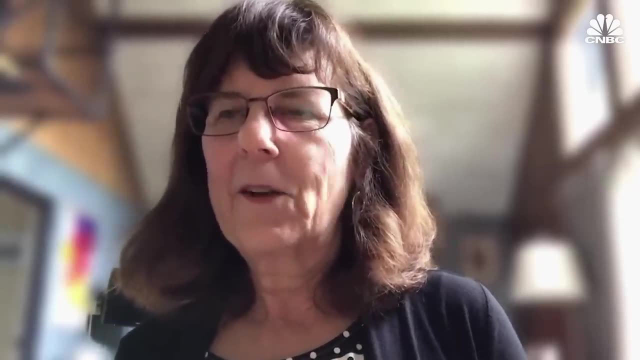 For energy in the US, but it's- you know it's- 1 percent, So you know it's helpful that everything counts And if you're going to be extracting the gas for other reasons, you might as well go ahead and do that, if you know if it makes sense from an economic. 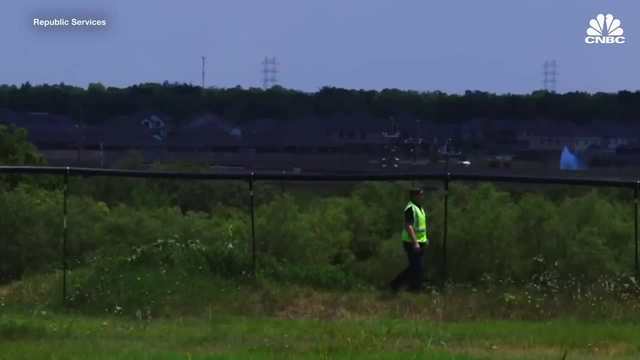 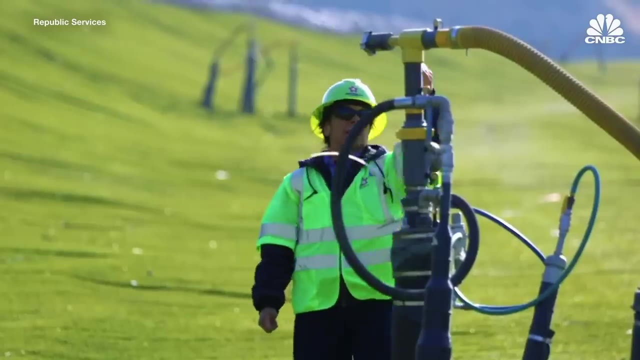 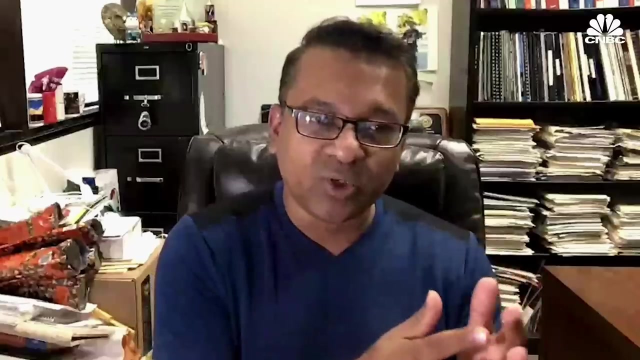 standpoint to generate electricity, But it's also a big investment. Landfill gas to energy projects can cost over $5 million to build and operate. While revenue from generating energy and fuel doesn't quite cover the cost, Landfills do benefit greatly From generous subsidies. many cities went into that landfill gas to energy. because they get the carbon credits and they get money from the federal government. when they are producing the gas and capturing the gas, they're converting that into electricity. The amount of gas you are capturing, you're reducing the greenhouse gas emission. That's why government was subsidizing, not only for carbon. 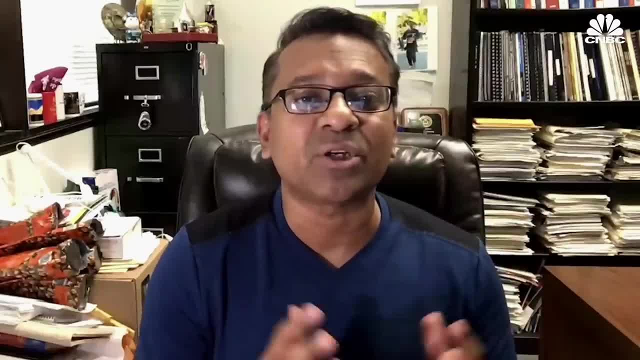 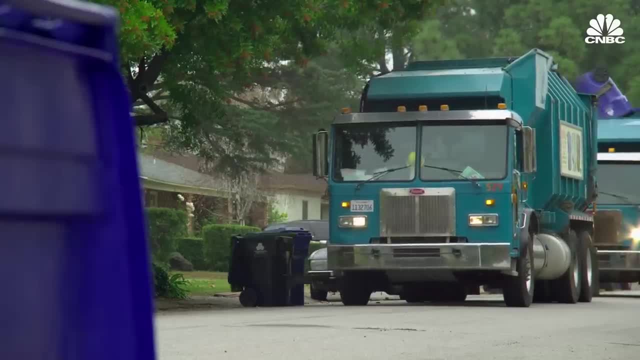 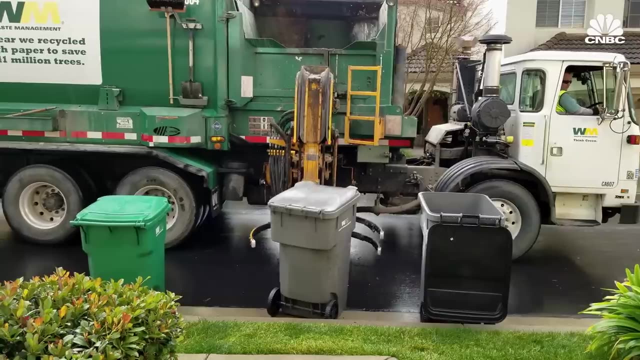 credits, subsidizing because you're reducing the greenhouse gas emission pressure on the environment. The tipping fee, combined with various mining techniques and government subsidies have together transformed the landfill industry into a booming business. It's a profitable industry. It's a difficult industry, but it is profitable. 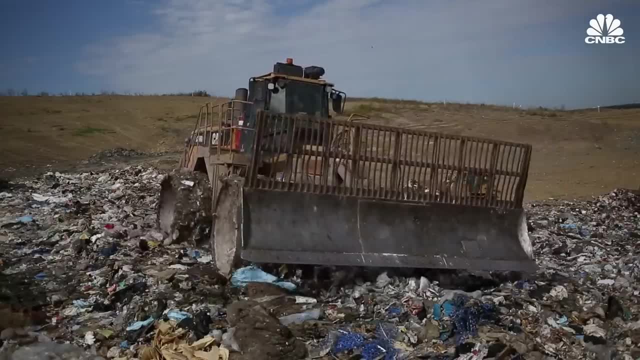 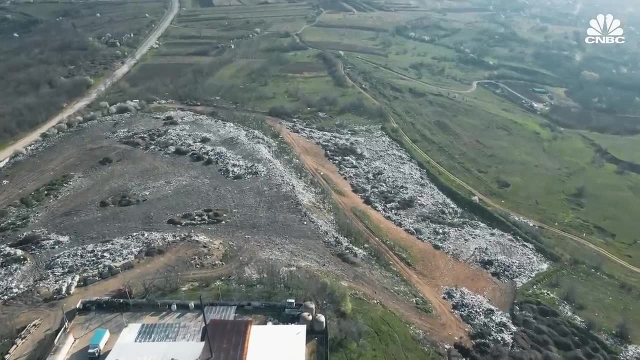 It's done right, And I think that is why there are so many private companies that are involved in waste management. Solid waste management will only continue to expand as long as there are those who view garbage as a resource rather than waste, Because when it comes to waste management, it's not just waste management. 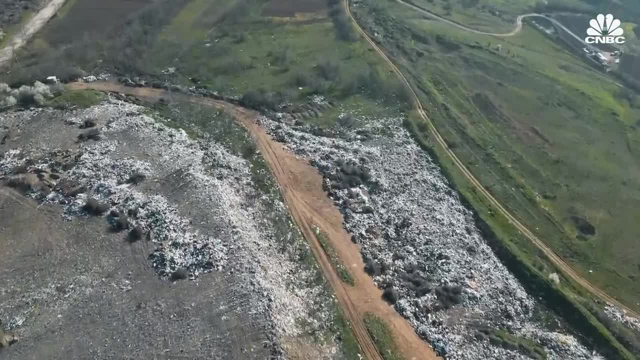 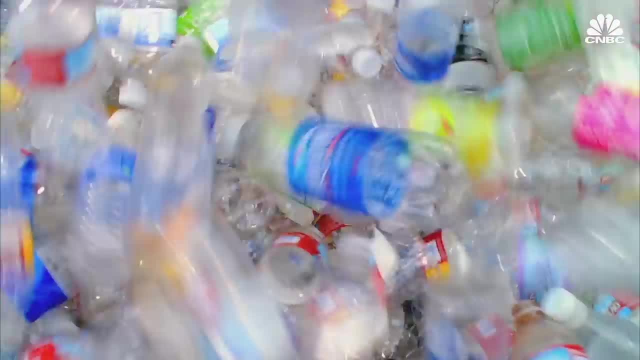 It's also waste management When it comes to landfills. one man's trash is quite literally another man's treasure. Waste is not a waste, but it's a resource, Because if you don't recycle the plastic, if we don't recycle the paper, if we 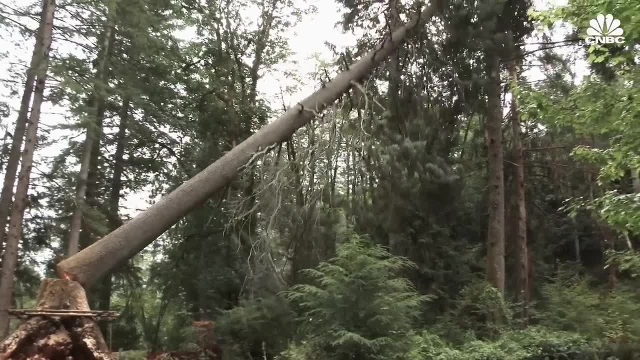 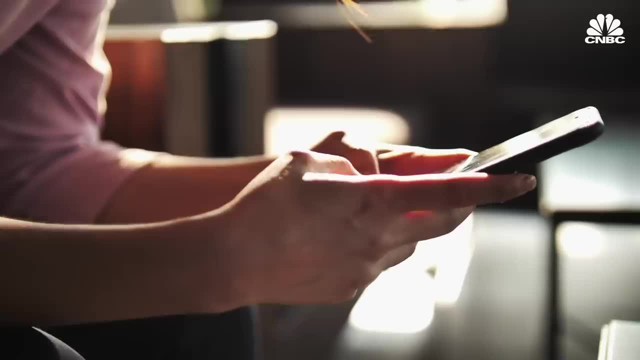 don't recycle the paper, what are you going to do? We are going to go and cut more trees If we don't recycle the plastic. we are going to go after more bio-products from gasoline If we don't reuse the electronic material. we are going to keep.